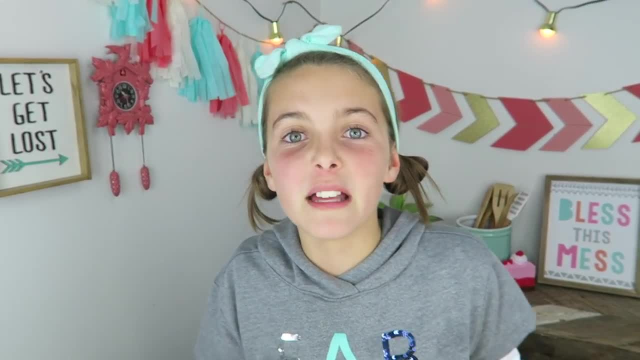 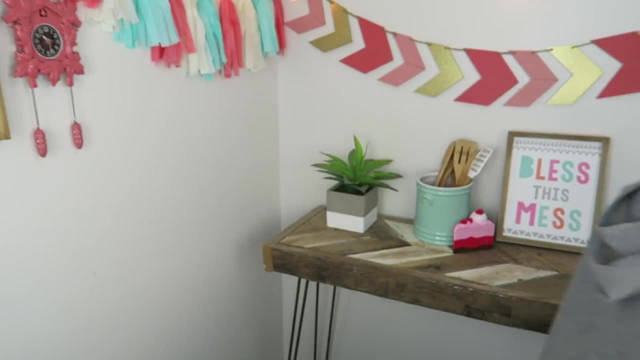 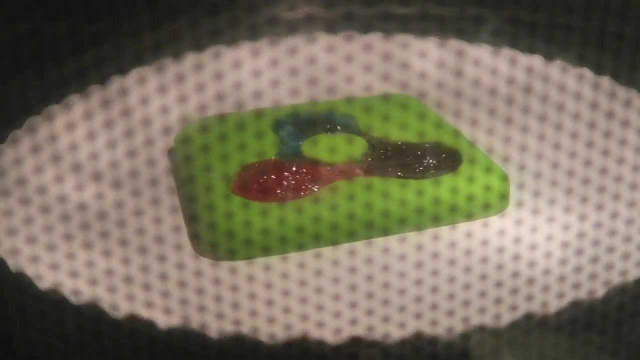 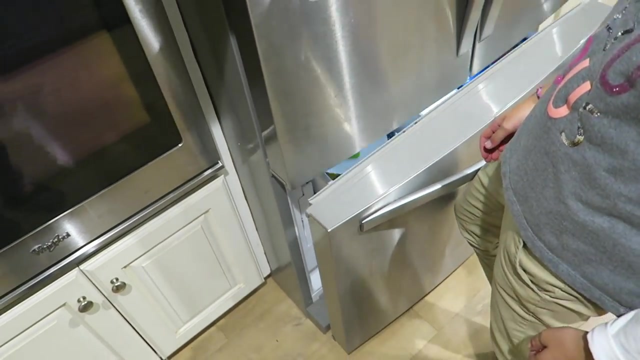 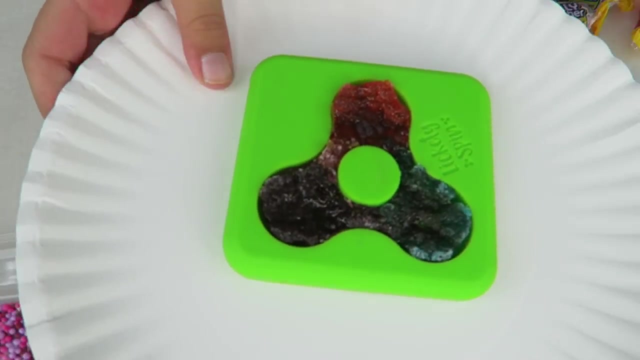 It's like cool. It melted perfectly, like this. All right, let's go. And then, when you get it out of the microwave, you put it in the fridge. It's ready. Look at this gorgeous thing. Oh, I can't wait to try it. It's all cooled. 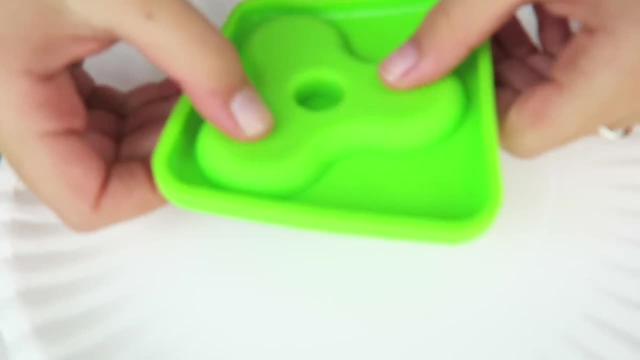 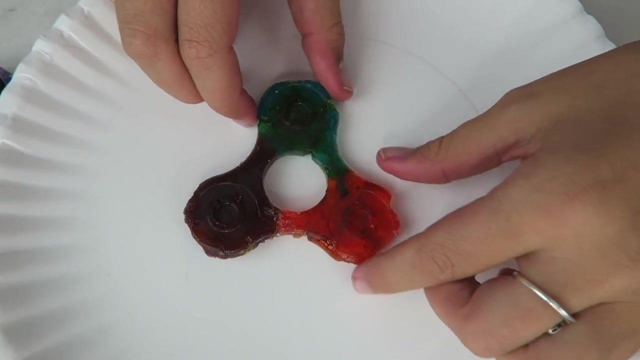 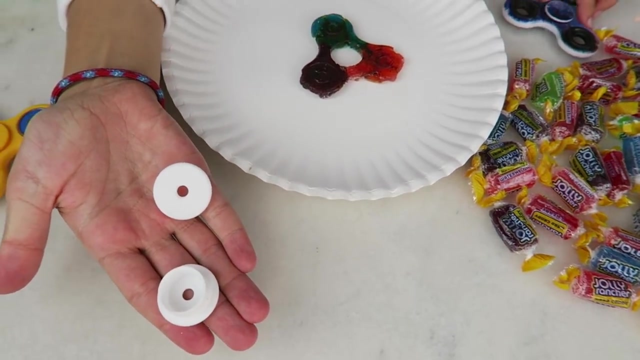 off, so let's pop it out. Just going to flip it over and press on each of the sides. Oh, look at that, It looks like a real fidget spinner. So in the package it comes with the middle bearing of a fidget spinner. 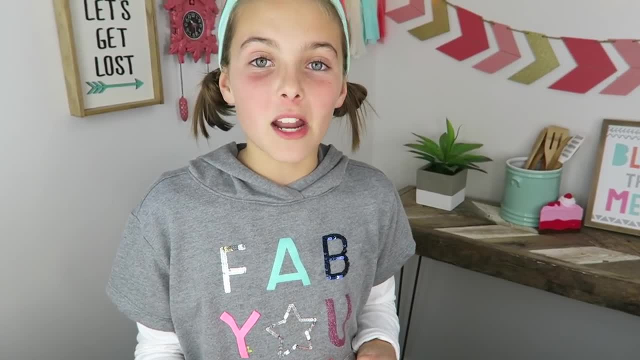 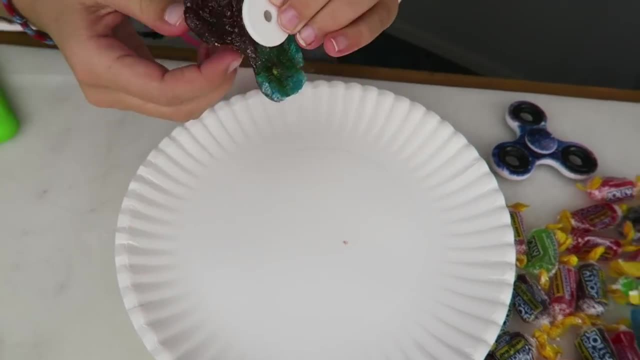 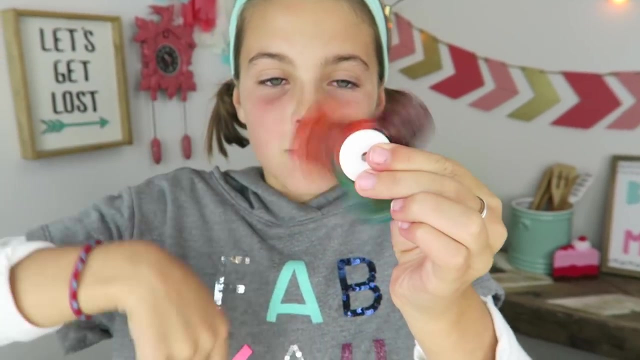 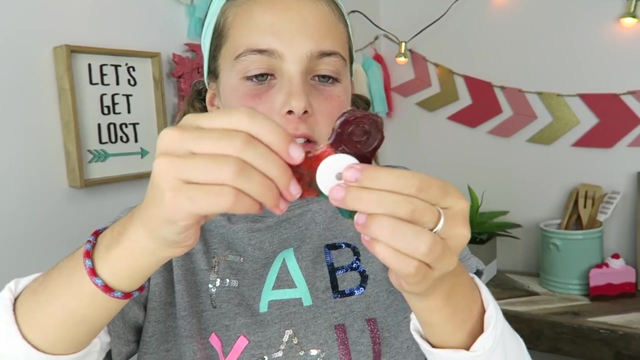 It's kind of like this part of the fidget spinner, but you get to snap it on in the inside of the candy. Pick it up and snap it on. Guys, look at all these cool colors. All right, let's test it out. Ready It spins. Whoa, I love the colors of it. 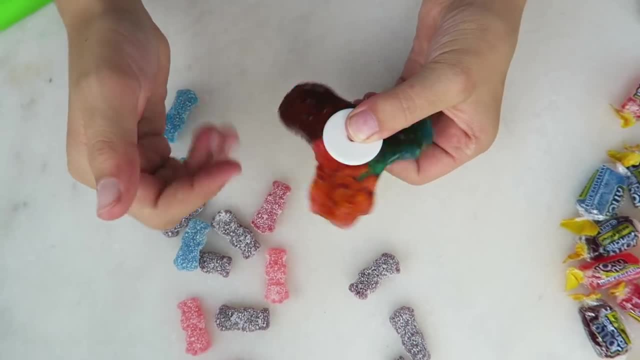 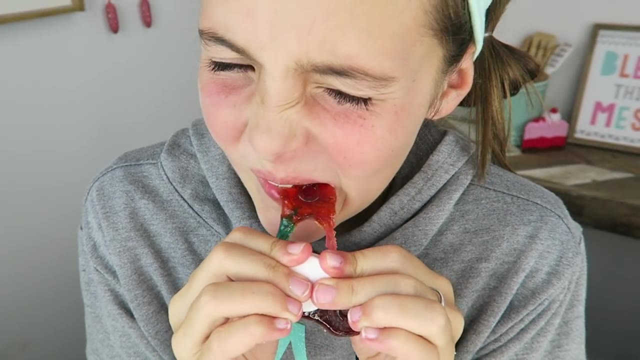 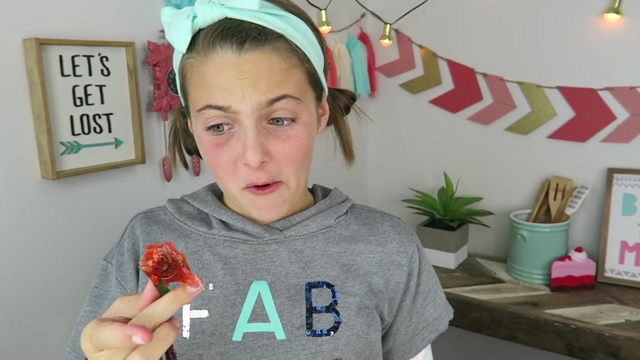 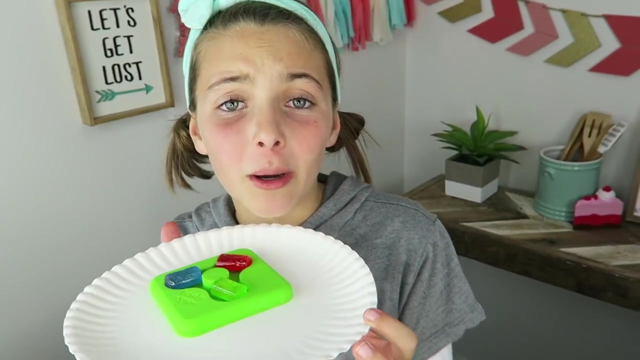 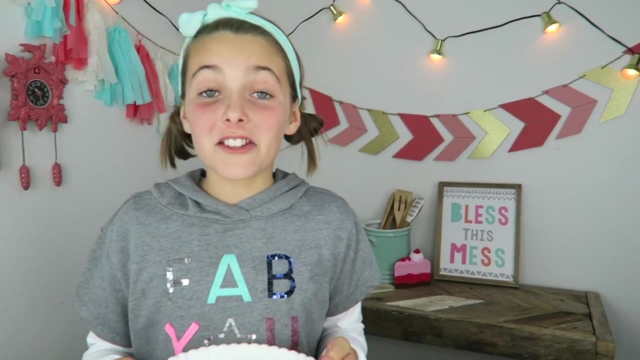 Okay, time to see how it tastes. Gummy, That's still really sour. Next is the Jolly Ranchers. I got them all ready, Now let's put them in the microwave. Okay, guys, this one turned out great. It's so smooth And the colors blended in with. 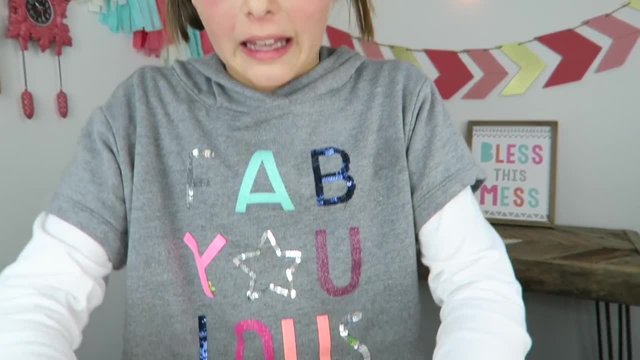 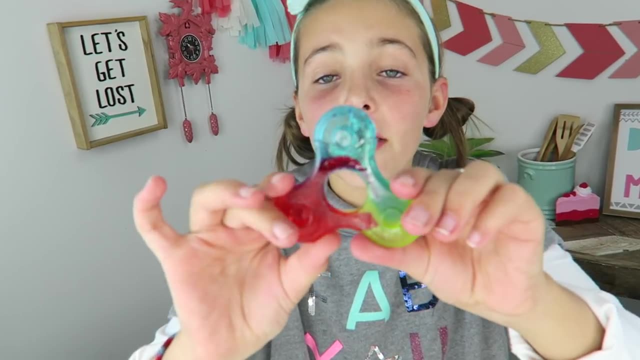 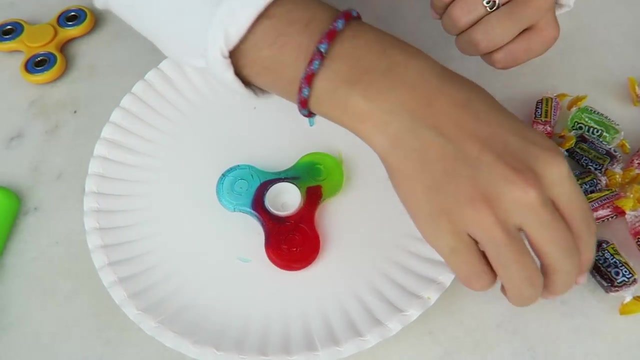 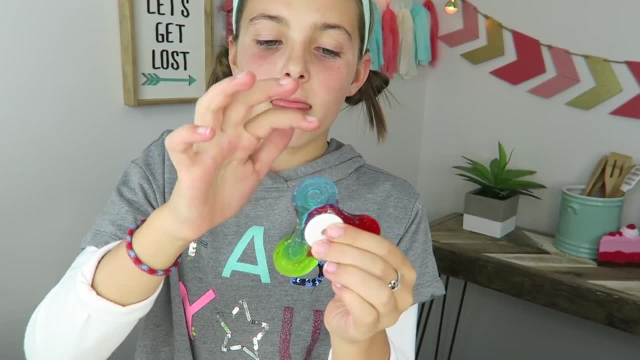 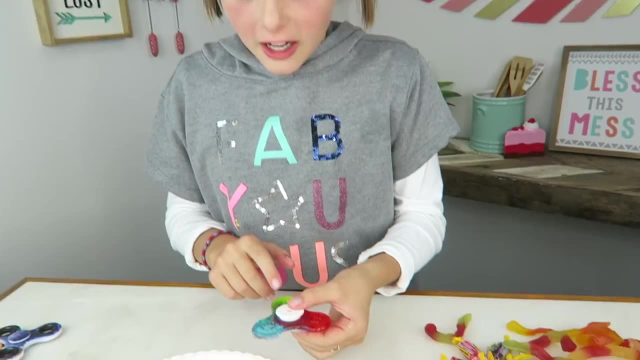 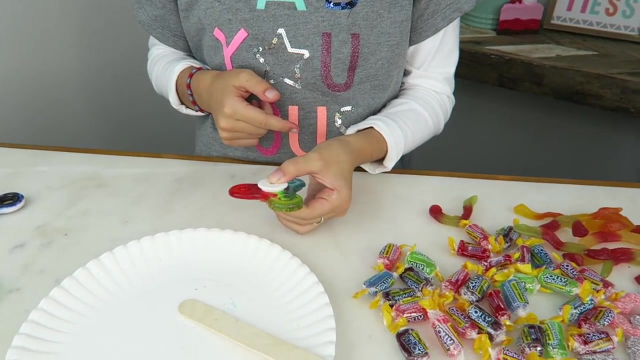 Okay, Time to see if it spins. Oh yeah, That is amazing Disco Party. I'm going to play a little game. Whichever color is closest to me or pointing at me, I'm going to try it. Okay, ready. 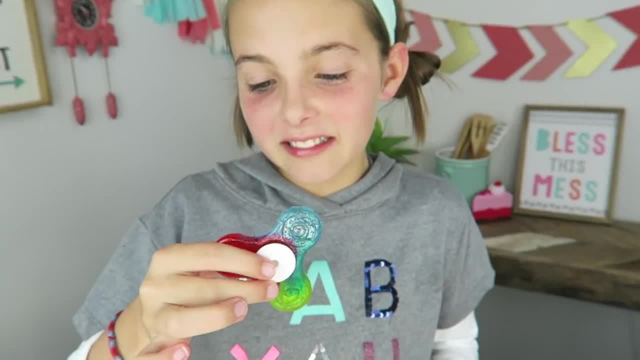 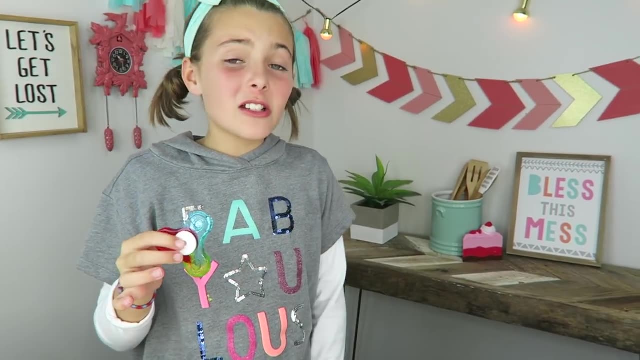 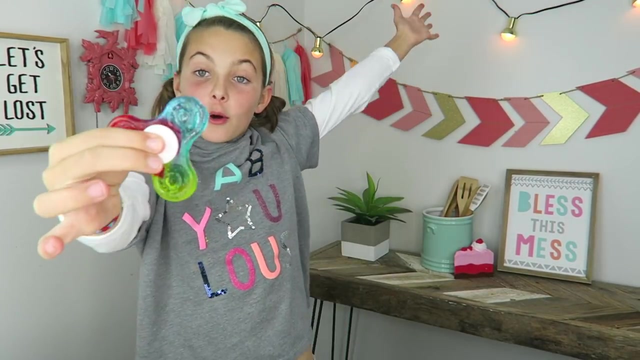 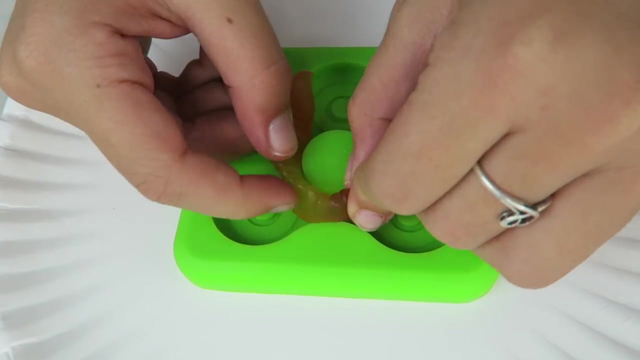 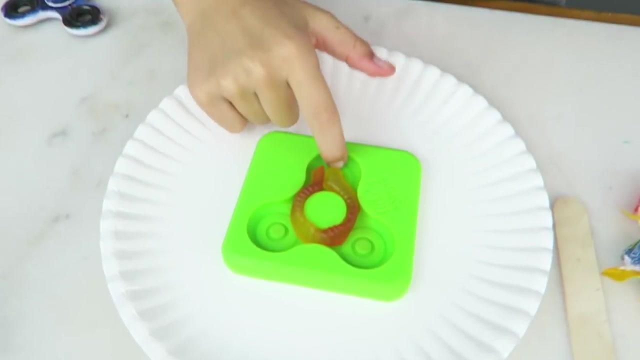 Blue, That's good. Red, I love this so much like you can just be walking around spinning your fidget spinner and then BAM, it's edible. okay, moving on, time for the gummy worms. I'm gonna like put this around the middle like that, and then I'm gonna rip this one up to each different. 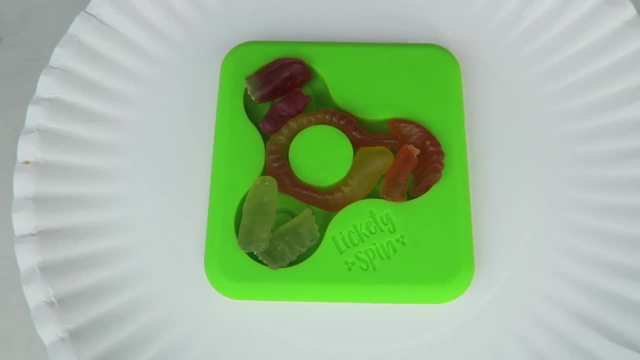 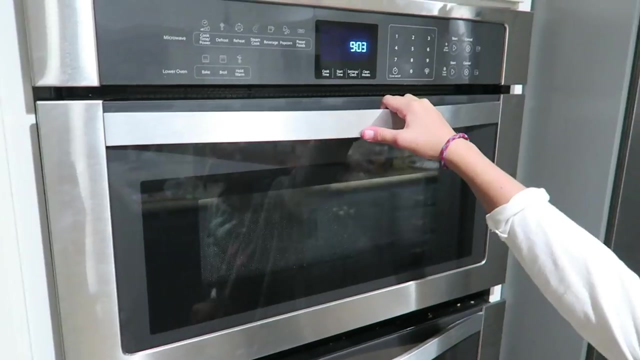 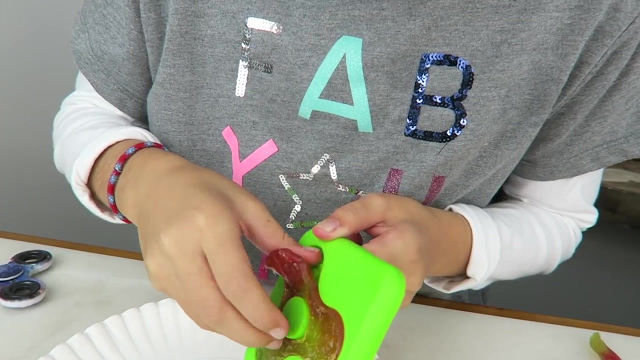 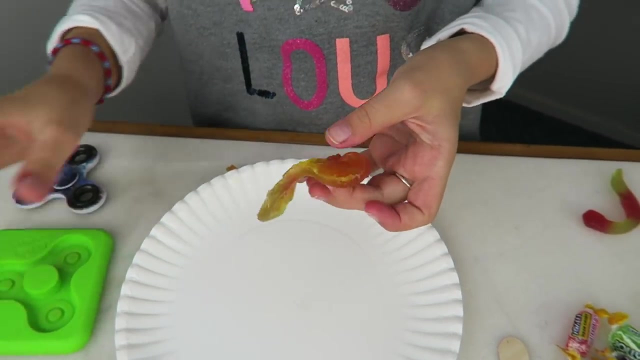 section: okay, wormies, time to go to the microwave. this one you kinda gotta peel. up there we go whoa peekaboo. okay, now I'm gonna put this one on the bottom of the bowl. okay, okay, I'm gonna put this one on the bottom of the bowl. okay, now I'm gonna put this one. 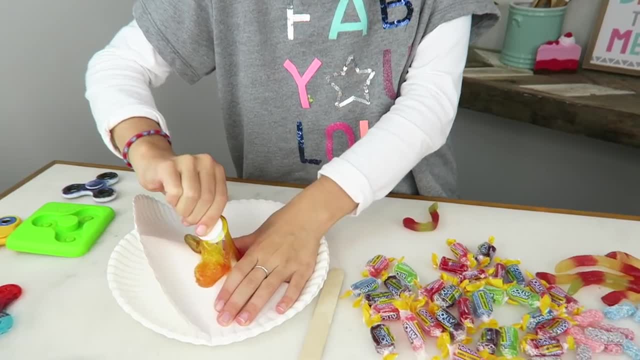 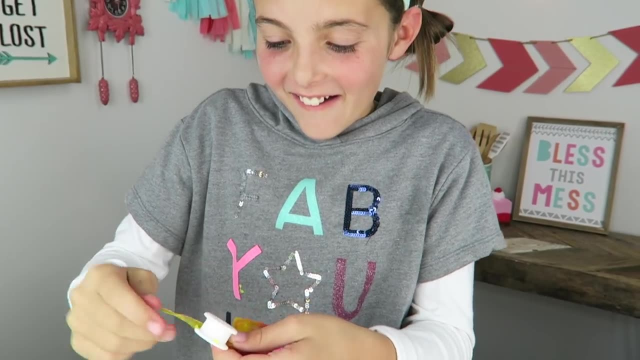 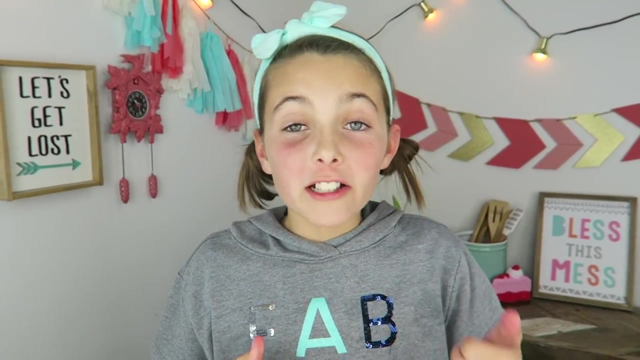 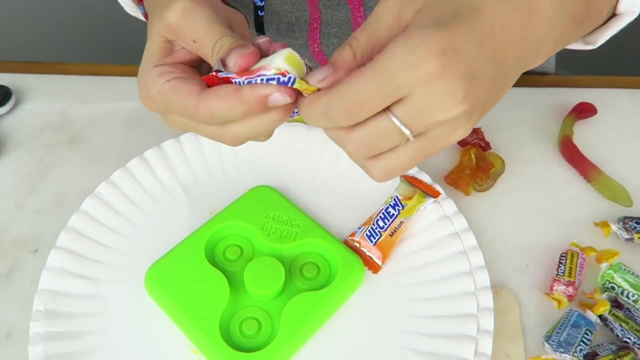 on the bottom of the bowl. okay, now I'm gonna put this one on the top of the bowl. okay, I'm gonna put this one on the main. broke it she — got it. What do you think? do you like it? What do you think, do you like it? 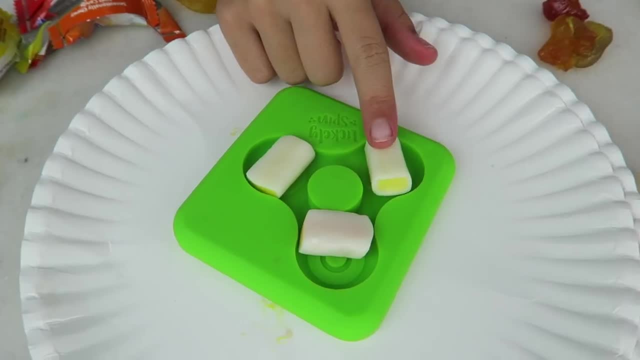 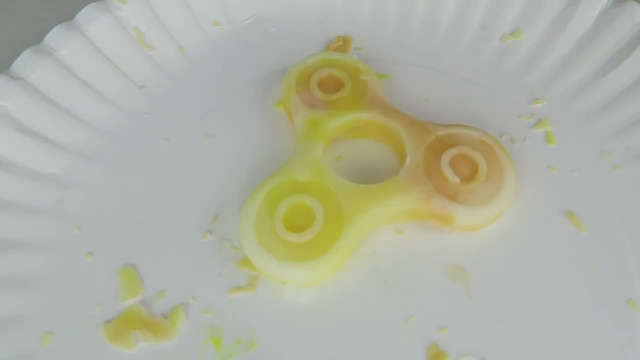 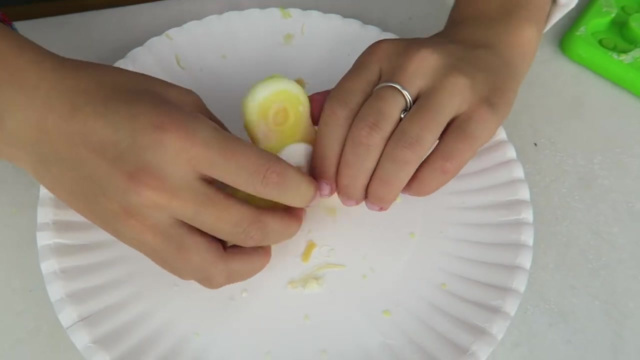 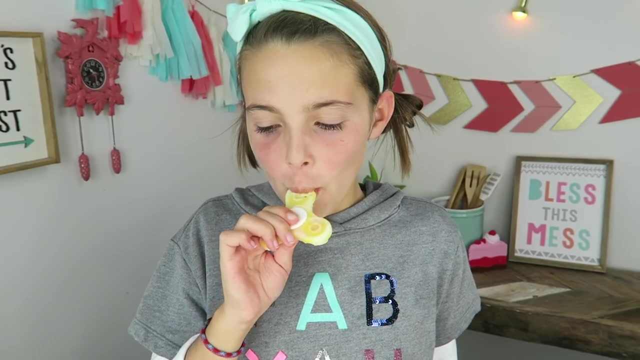 Do you like it She —. she said yes, saying yes, Banana melon. All right, let's put it in the microwave. Whoa, that looks cool. There we go. oh yeah, Okay, I'm gonna try it, Mm bananas. 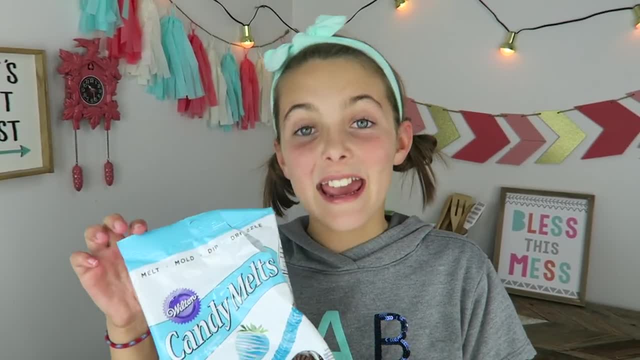 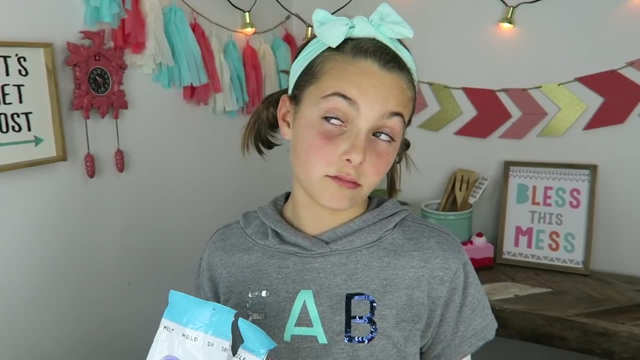 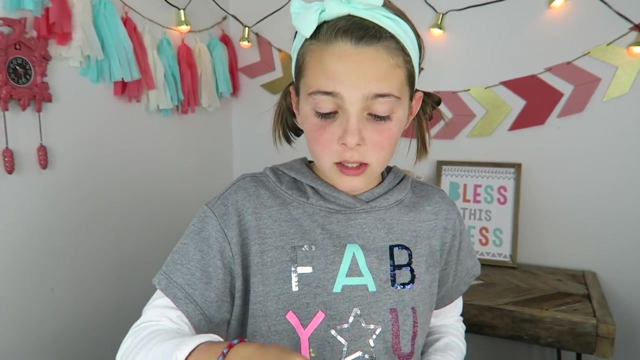 Okay, we have a bonus round for you: Candy melts. It's kinda like chocolate, but it's not, So I already have my candy melts melted here, So all we gotta do is just pour it into the mold and then pop it into the freezer.